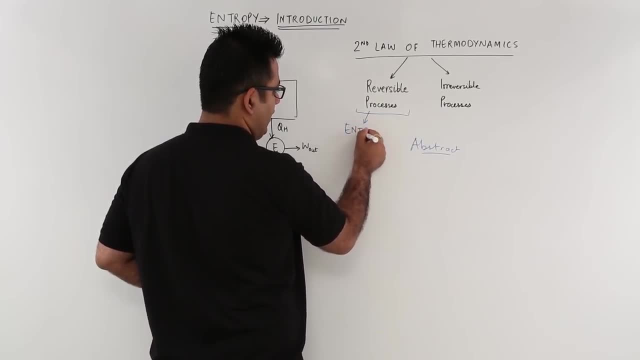 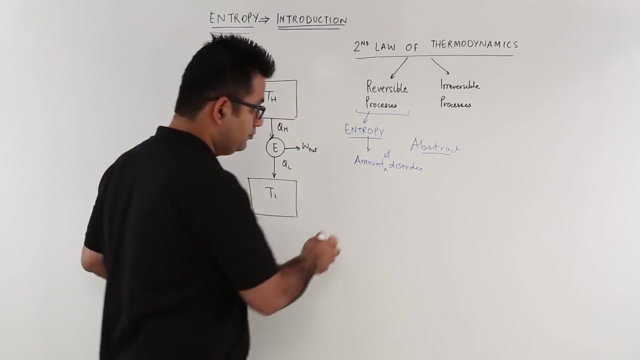 So we study entropy in context with the reversible processes only And to define it you can say in a very simplistic manner: entropy is the amount of disorder, amount of the process, Nh or truth. in context of the third window You can write it as the loss of cause in. 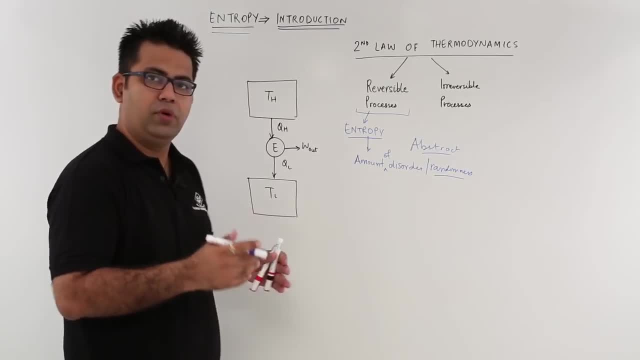 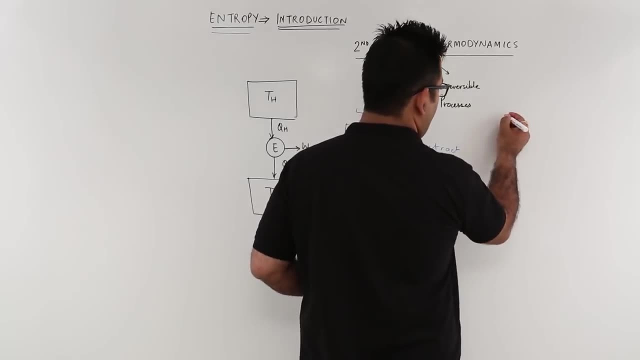 the basis of lifetime. So if you have the stress order which is just equal to this particular product, which is the loss of structure of the material, which is check, if you have any group of very simple properties, So we define then the, the relative stress on which this 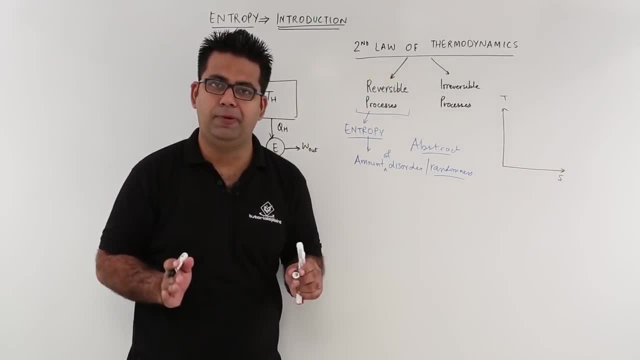 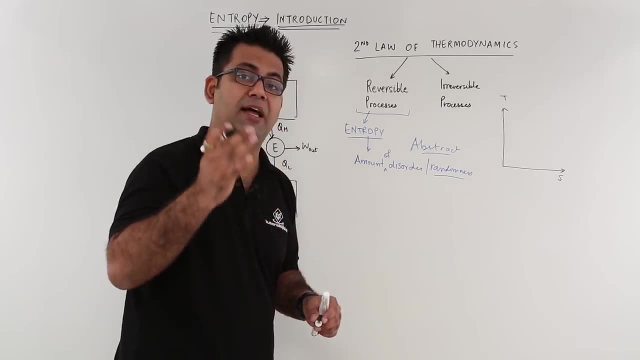 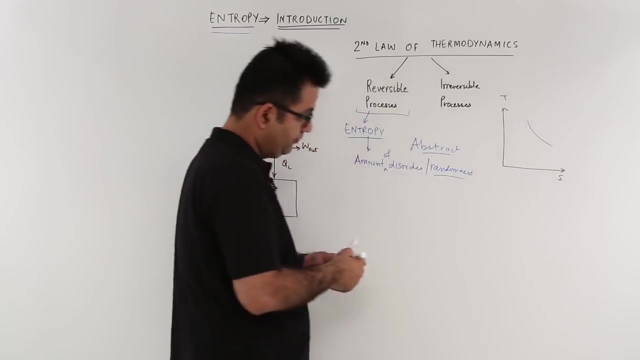 Okay, if we are not talking about isentropic processes wherein the entropy remains same, let us talk about compression and expansion, which are not isentropic. Okay, let us say you have a certain process which is going like this. Okay, now what is happening? 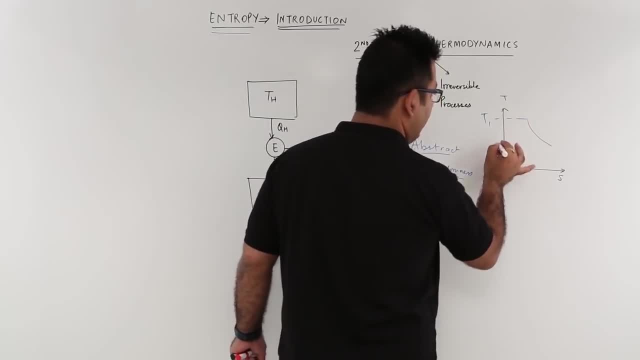 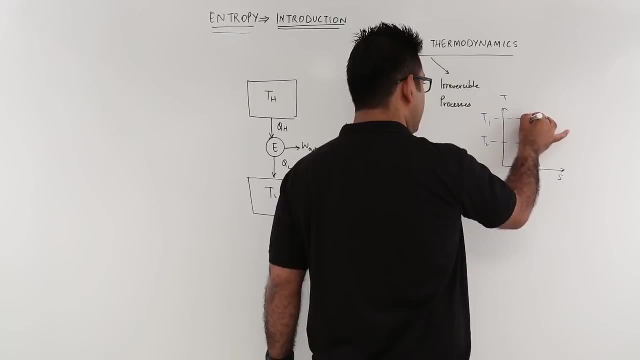 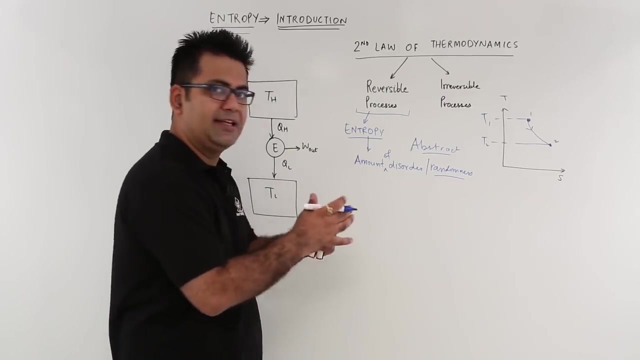 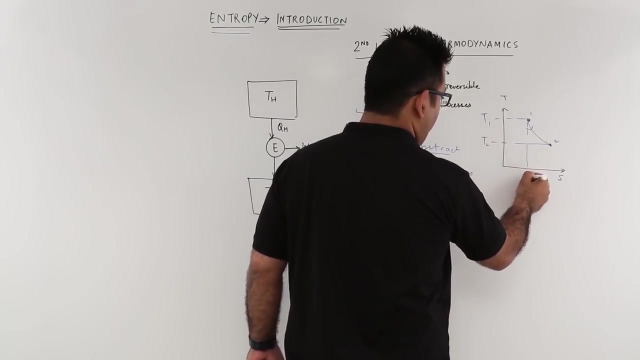 Initially you are at this state, that is T1 and the final state is T2.. Now the temperature has gone down from T1 to T2.. Now temperature goes down. when the gas expands, It decreases in temperature. Now what happens if you look at the entropy? 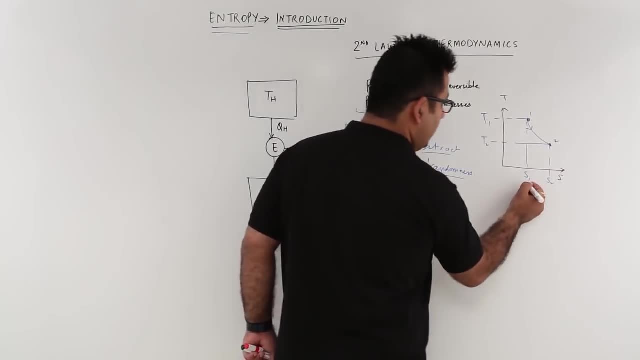 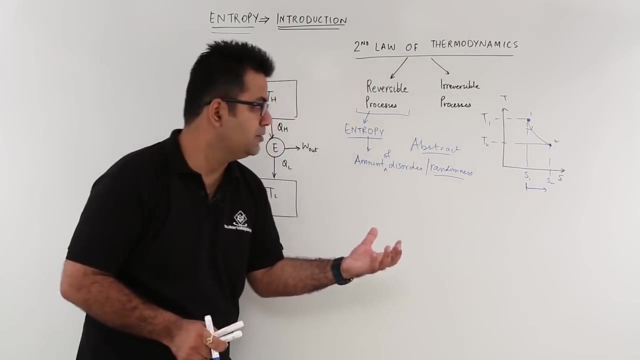 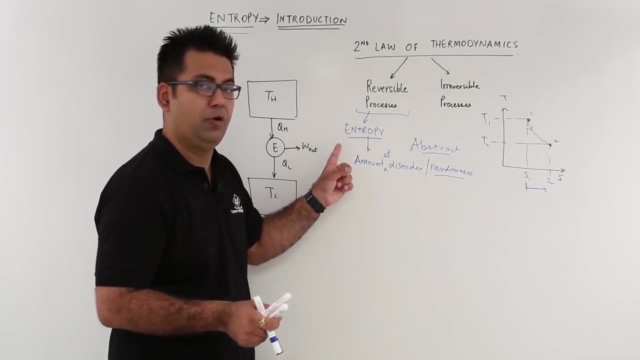 The entropy has increased from S1 to S2.. Now, in a very simplistic manner, if you understand this in physical terms, as we told you, that amount of disorderness or randomness of the molecules of a system is the entropy or is the measure of entropy. 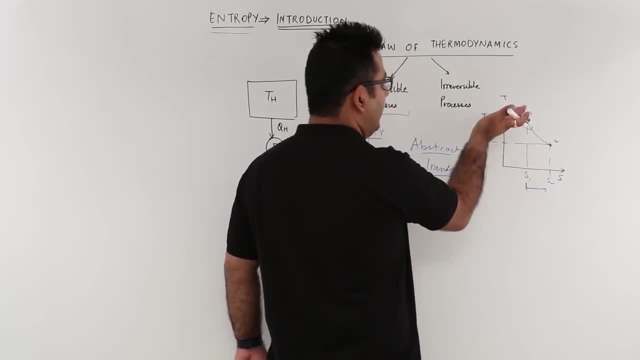 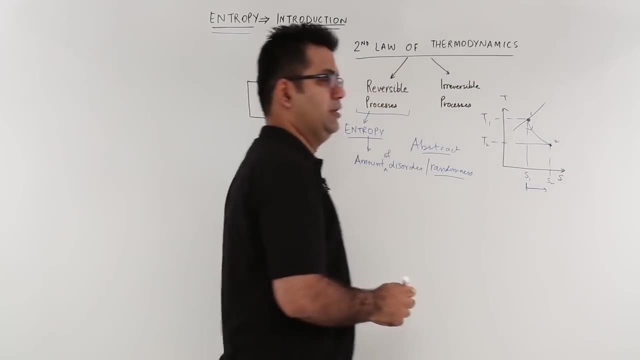 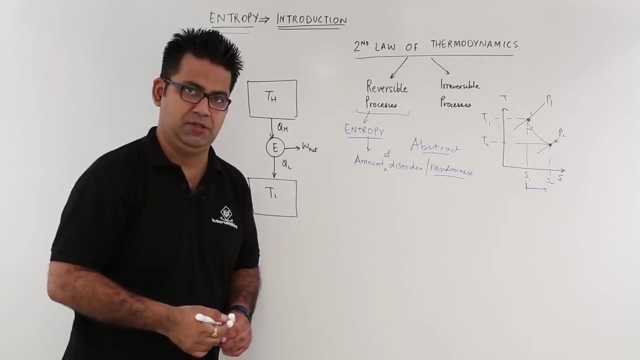 Okay, if you take this at higher temperatures or at higher pressures and if I draw an isobar, this is a constant pressure line and this is also a constant pressure line for P1 to P2.. So when your pressure drops from P1 to P2,. 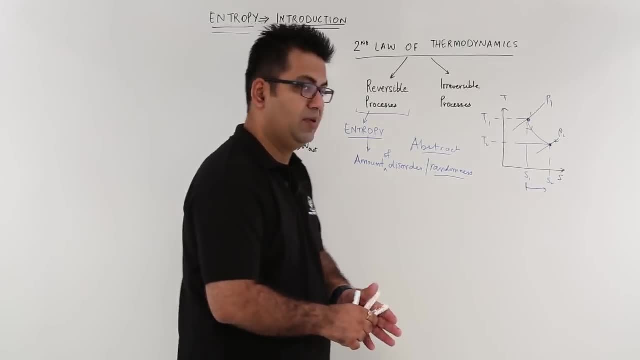 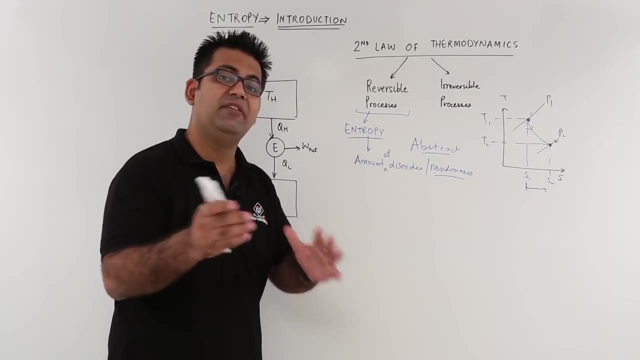 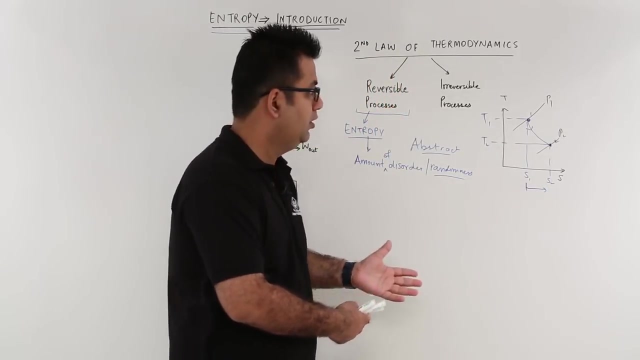 which will give a rise in the volume. Okay, so as the volume increases, expansion takes place. the randomness of the molecules will increase. On the vice versa part, if you compress the gas, the randomness would decrease, so the entropy would decrease. Okay, so this is a very, very easy method of understanding entropy. 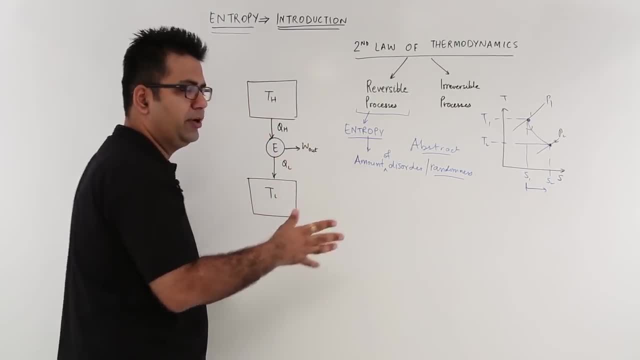 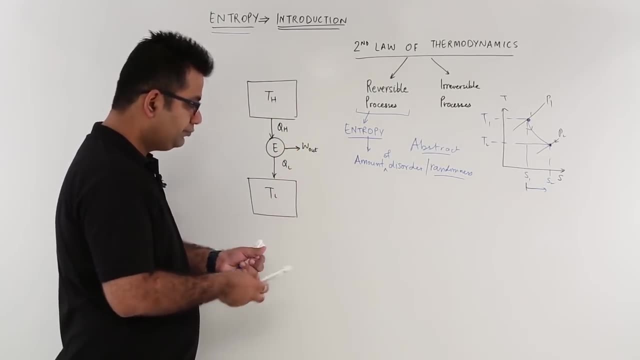 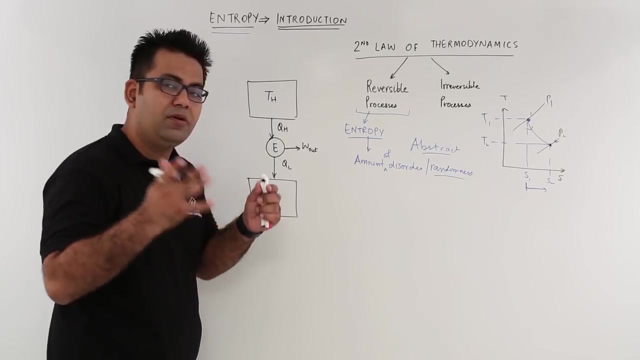 Okay, now let us talk about it in the context of second law. Okay, now let us talk about it in the context of second law. We will be dealing with lot of heat engines, heat cycles. If you look at this heat engine, The amount of work that comes out of a heat engine- 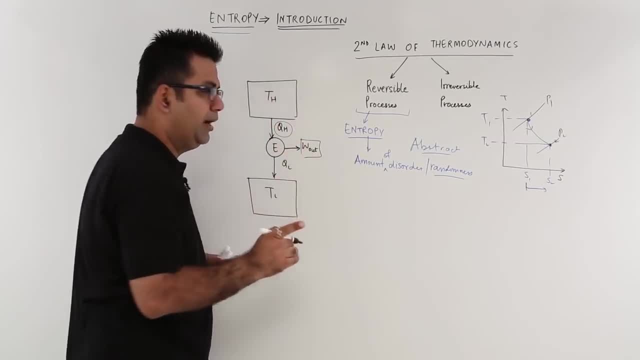 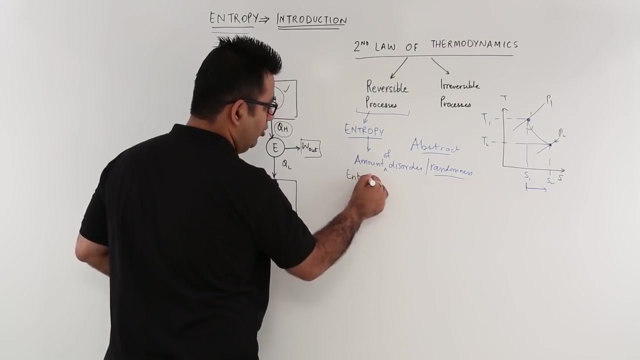 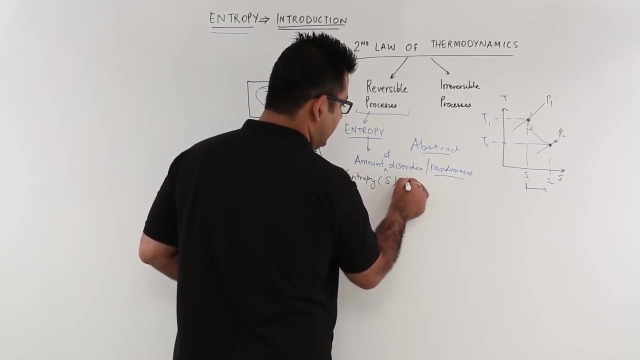 is not a function of the amount of heat supplied. It is a function of, or depends upon the temperature at which the heat is supplied. Okay, So this means that the entropy we will denote entropy with capital S. so entropy basically depends upon or is: 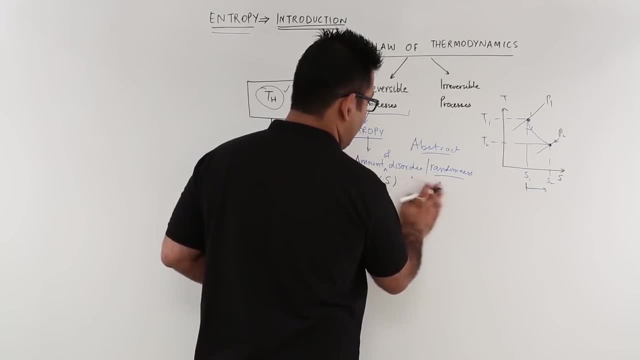 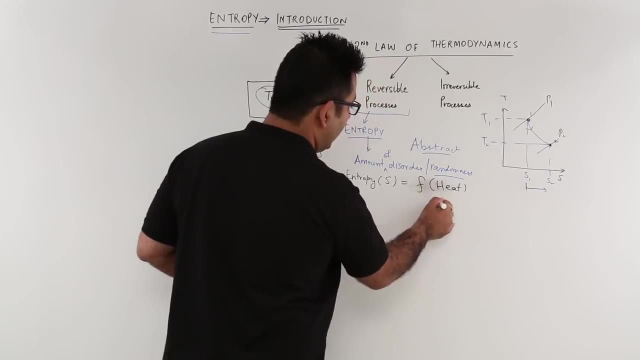 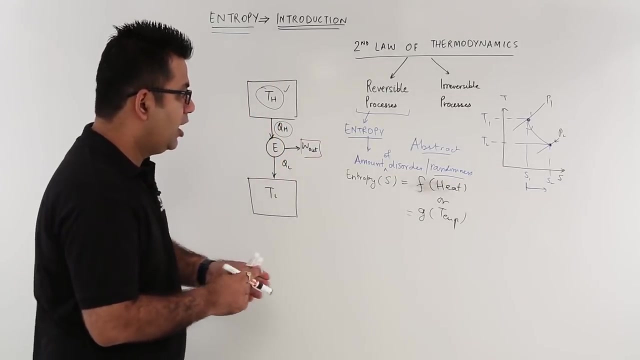 a function of heat, depends upon, or let us say, is a function of heat, or I can say it is a function of temperature, because how much heat is being supplied is dependent upon at what temperature it is being supplied. so we are more concerned with the temperature at 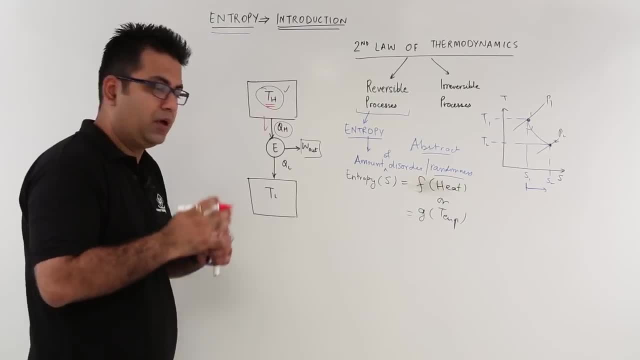 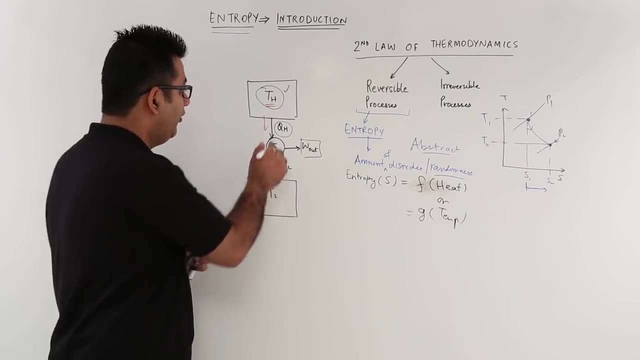 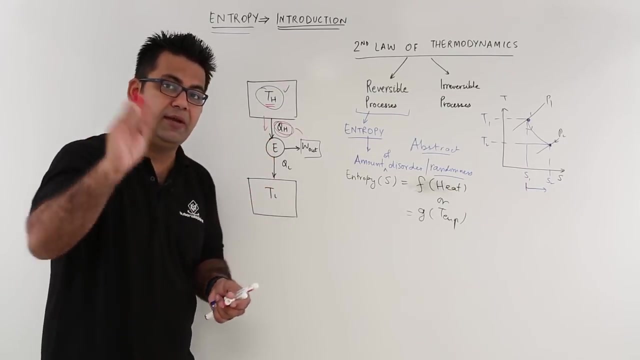 which the heat is supplied to the engine. because higher the temperature at which the heat is supplied you have more chances of conversion of this heat into earth means your efficiency would be higher. So if you supply heat at a lower temperature you have less chances of that heat to be converted. 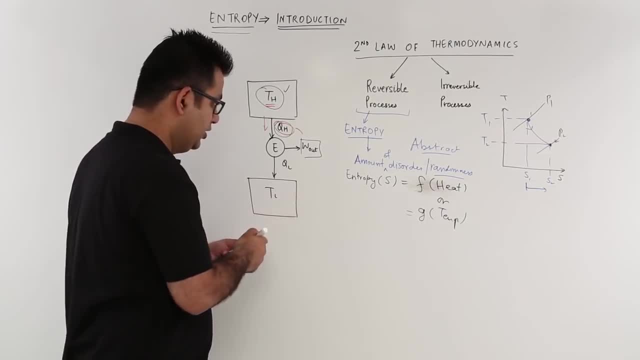 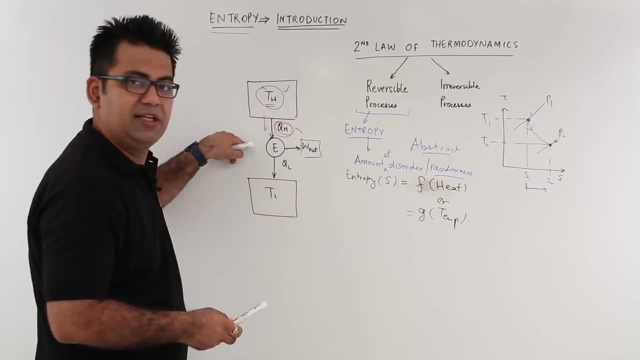 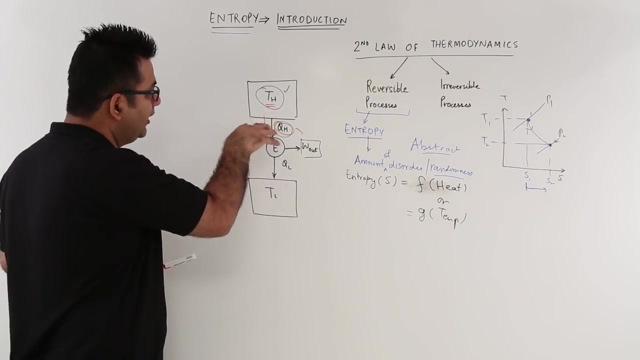 into some amount of work from that engine. so if you are supplying heat from a very high temperature to this engine, the entropy increase would be very, very small. on the other hand, if you are supplying heat to this engine at a very low temperature or comparatively low temperature, 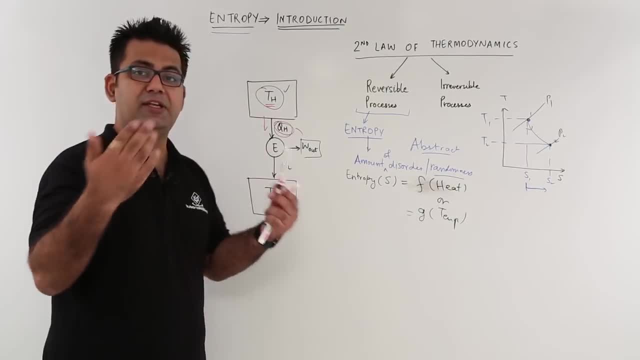 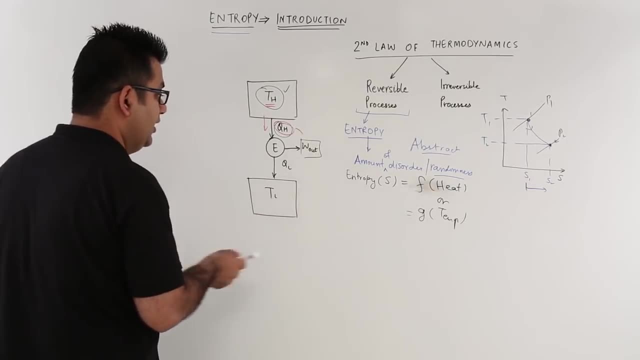 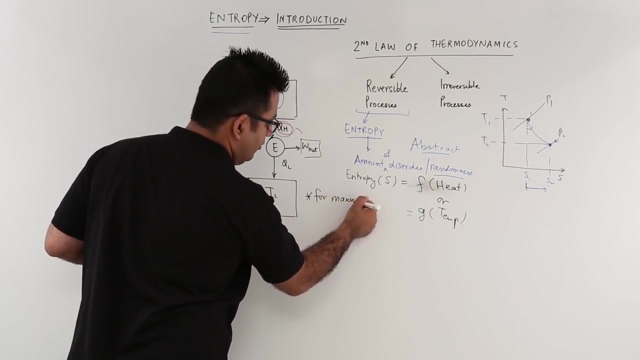 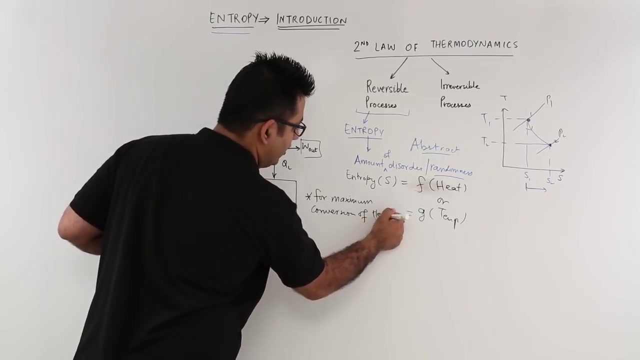 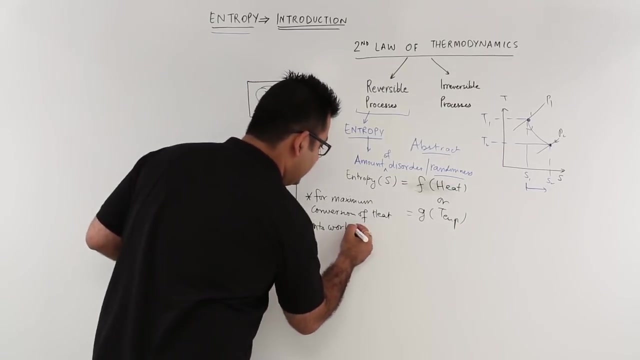 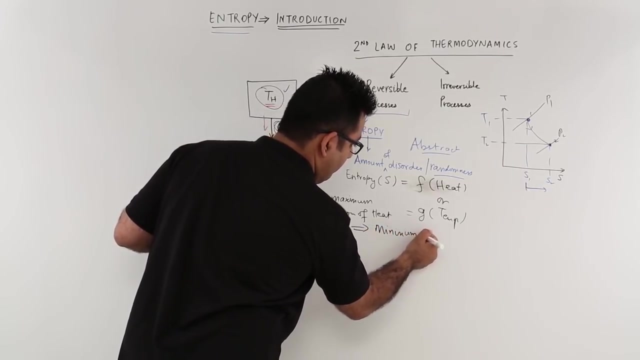 Then in the previous case, then your entropy change or your entropy increase would be very, very high. so this brings us to a very important observation over here: that for maximum conversion of heat into earth, Maximum conversion of heat into earth, heat into work, this is associated with minimum entropy change. minimum entropy change or entropy.